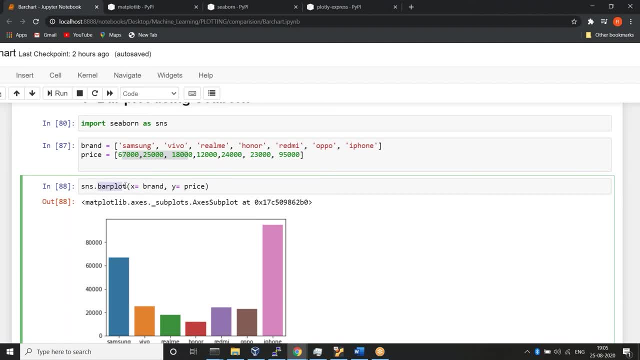 and based on that, I'm just giving SNS dot bar plot. So this is pretty much straightforward. So this is your library. in that library I have something called bar plot by you using that. I'm just mentioning x-axis, brand, So which is this, and y-axis, which is price. 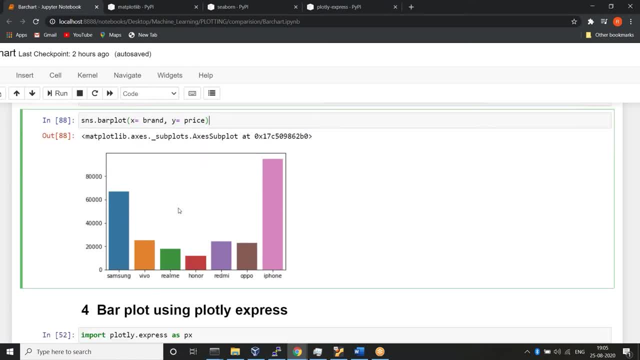 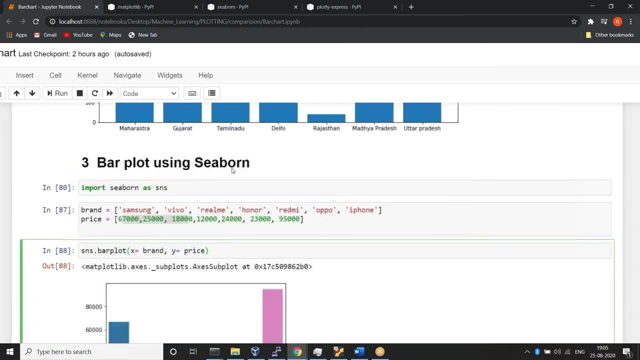 So that's how I'm able to get the bar plot. So this is how you'll be able to get. but inbuilt seaborn is having some themes, So that's why this plot looks better when compared to matplotlib, And let us understand plotly Express as well. 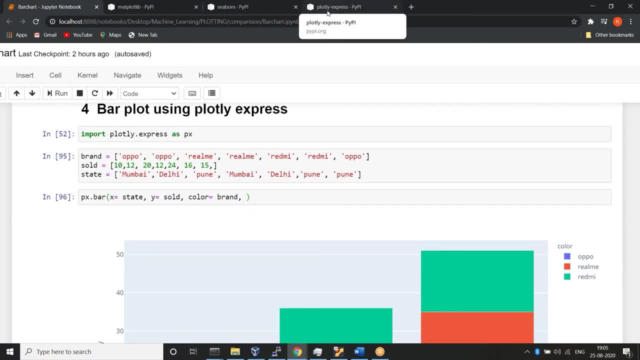 So before that I have already said: just go and download plotly Express, So in pi pi. so just copy and paste it in your Anaconda prompt. So import plotly dot Express as PX, and after that I'm just taking it as brand: how many, how many they have sold like. 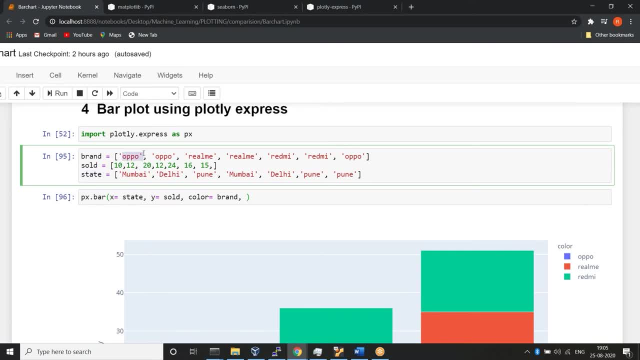 like each state, how many, how many they have stole, based on the brand. So let's assume, oppo, They have sold 10 in Mumbai. in Delhi, They have sold 12 pieces on Oppo in Delhi. So so, likewise, I have just taken some sample data and then, based on that, 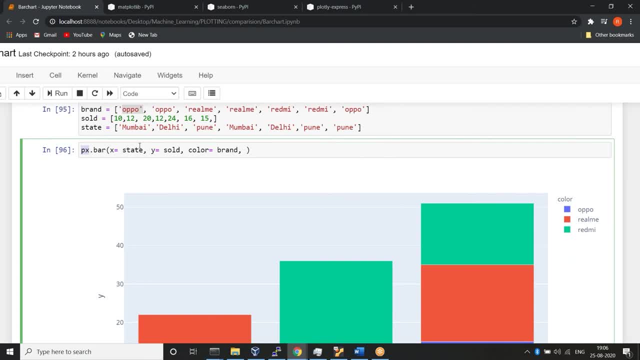 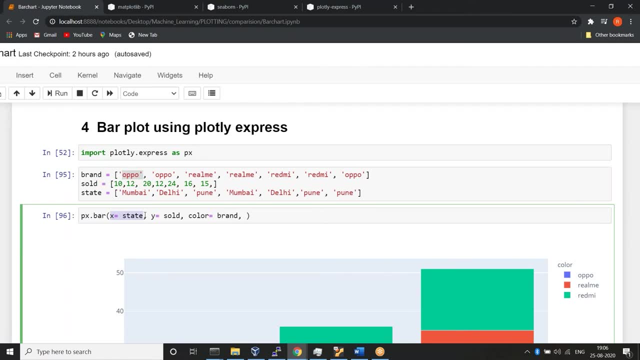 So what is this PX dot bar? So PX is nothing but your plotly Express and dot bar- and here I'm just mentioning x is equals to state, So which means this, and y is equals to sold, So this one. and then color is equals to brand. 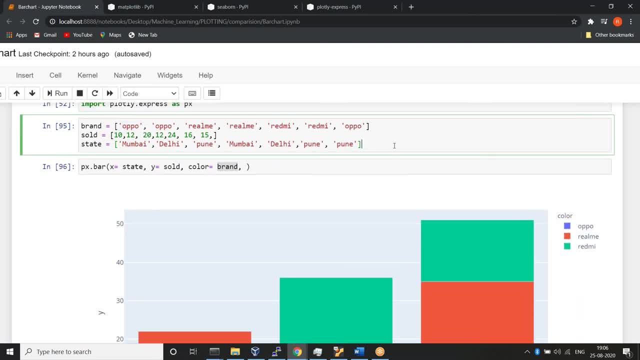 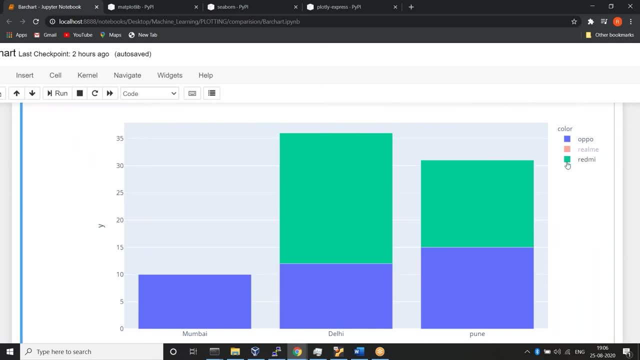 So, based on the brand, I can just shift it. So how, let us? let us understand that as well. So just simply execute that and just click real me, and then, if you don't want that, you can just go with only Oppo. So this will be pretty much interactive. 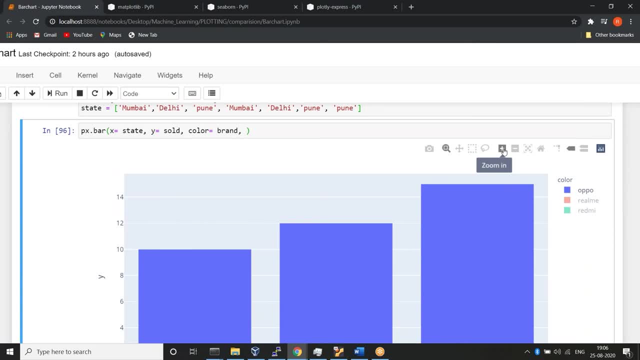 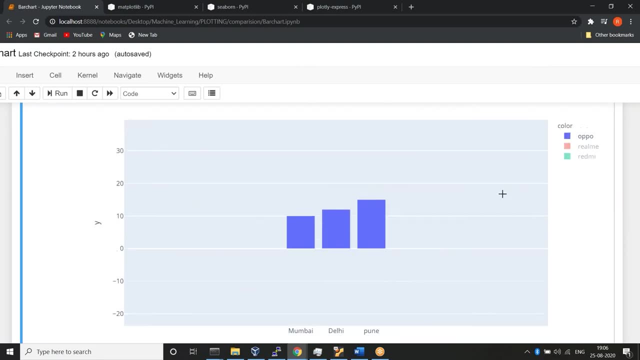 and here you will be having more options over here. So if you just click zoom in, so it will be, it will be zoomed in and after that you can even use zoom out and even more, even more. and if you want to just auto scale, just type auto scale. 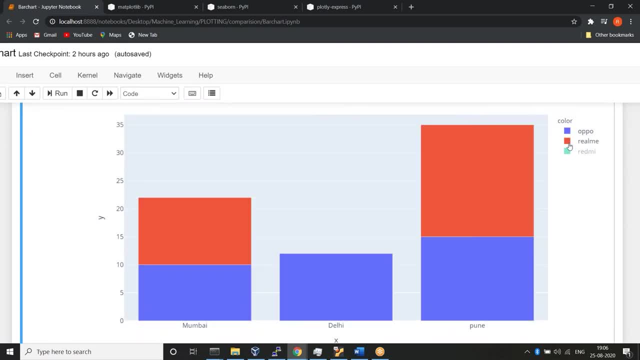 and again it will be back to normal. if you add real me, Yeah, I will be able to get and you can clearly understand. for Delhi, So how many pieces I have sold. so Oppo, which is Delhi. So, if you are able to see here, so color is Oppo and x-axis Delhi.